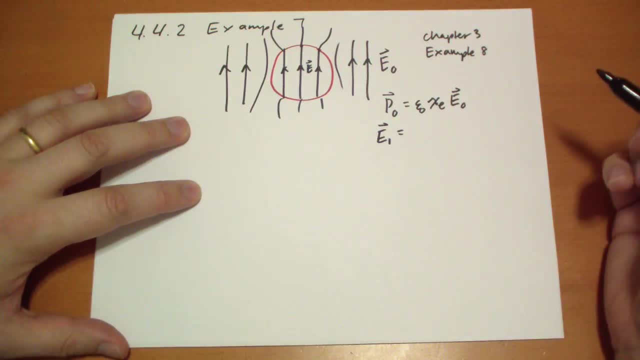 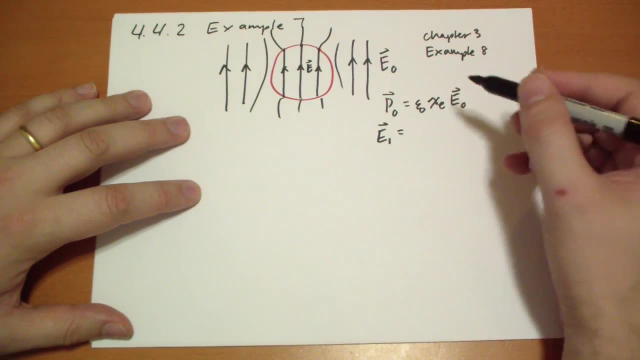 So I'm going to call this. E-one is produced by the polarization. We solved this problem Back in example two of section four. two one- we get negative one over three epsilon-naught of the polarization that we just produced. 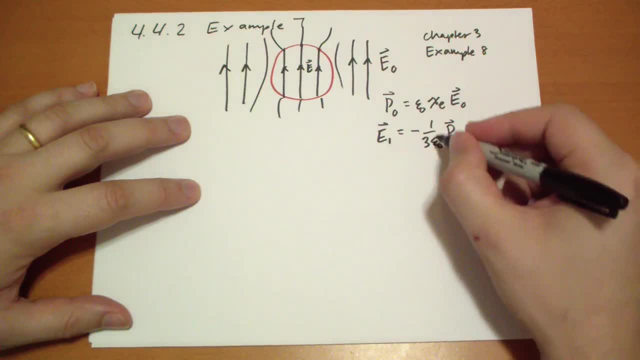 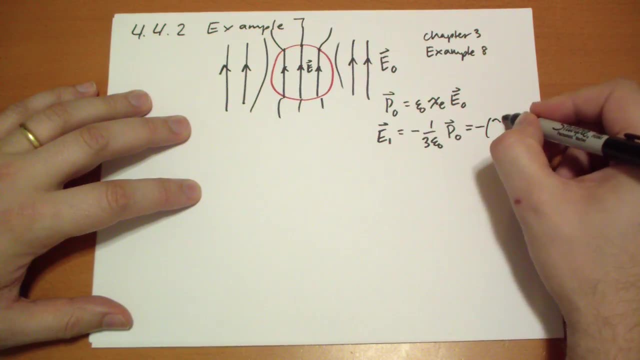 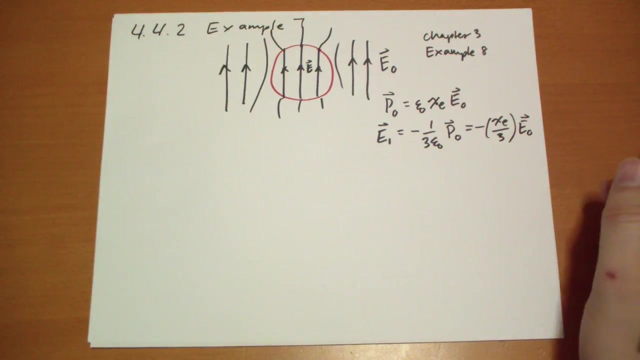 Okay, And that's going to be equal to plug in this original term. here or there we get minus chi-E over three, the susceptibility divided by three of the original electric field. So if you were to see what this new electric field would produce in terms of polarization, 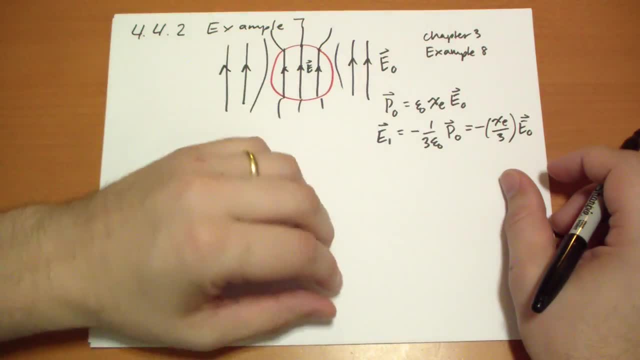 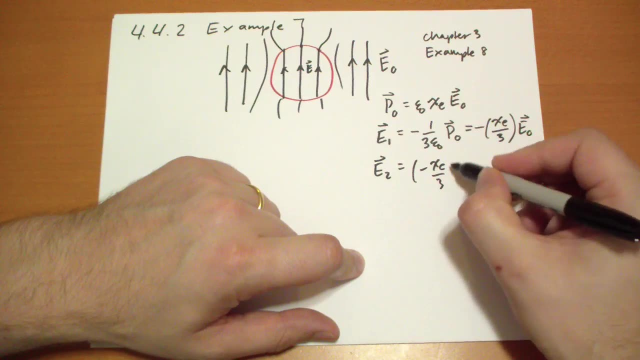 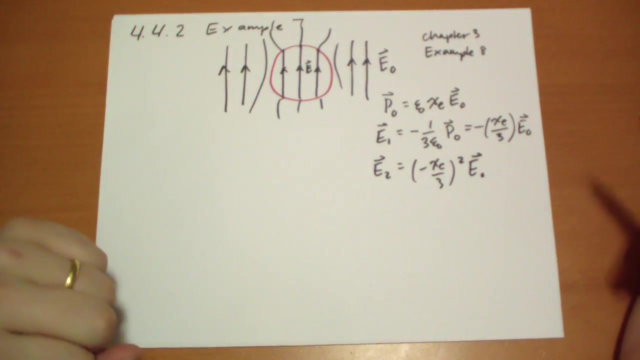 and what the resulting electric field from that new polarization would be. you just basically do what you just did and you end up with negative chi-E- over three squared times the original electric field, And the idea is that you're going to add up all these fields on top of each other. 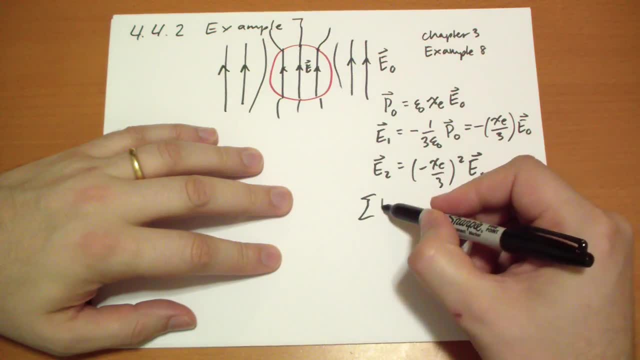 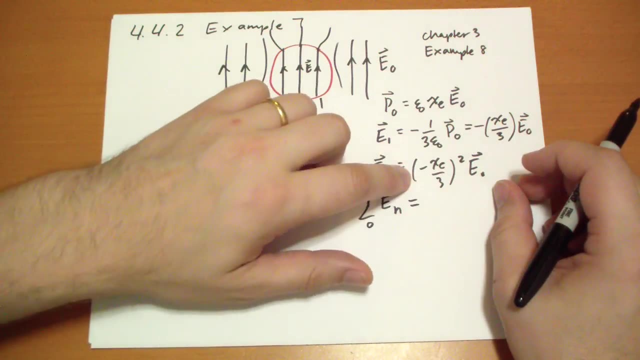 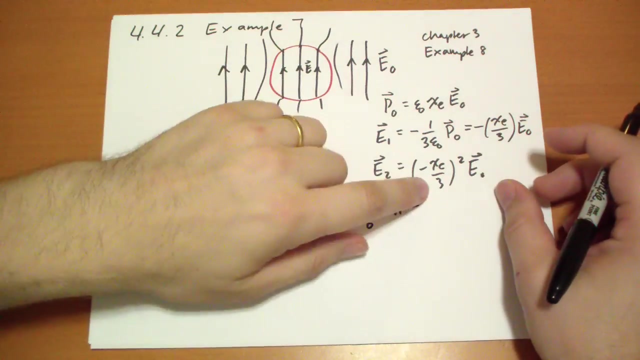 using the principle of superposition. so we're going to take the sum of all these electric fields from 0 to infinity and we're going to get some answer. now, looking at this, this is a geometric series where the number itself is less than one, so we can just apply. 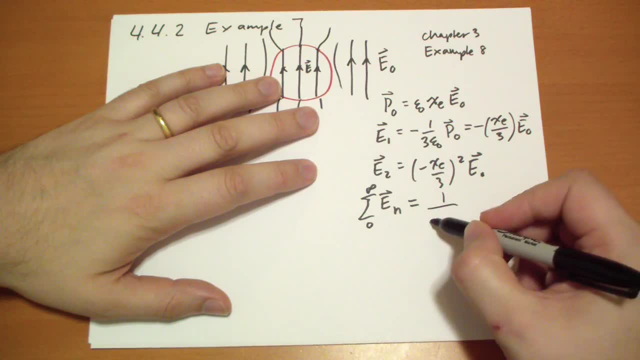 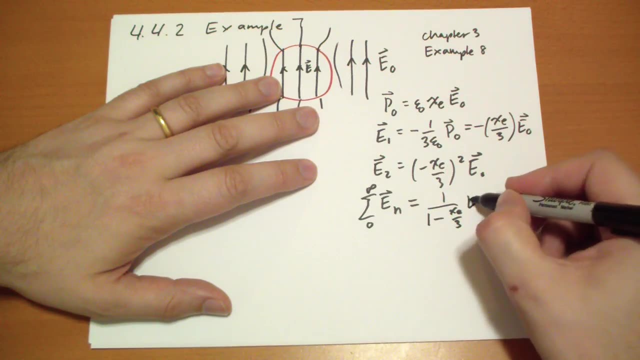 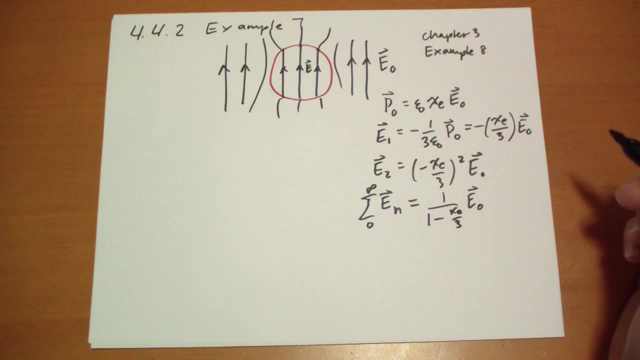 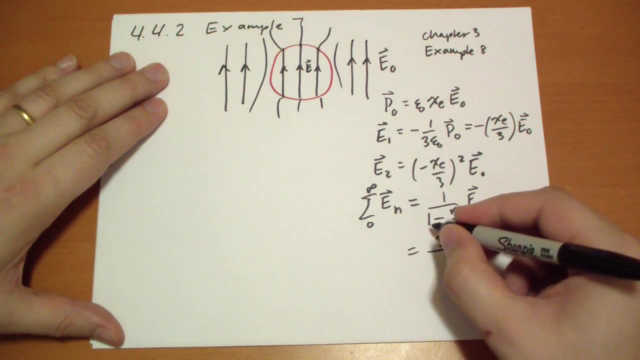 the simple rule that this is equal to 1 over 1 minus chi e over 3, the thing that we're taking the exponential of times the electric field, that's the geometric series result there. so another way to write this could be: you multiply top and bottom by 3 and you get 3 minus chi e. 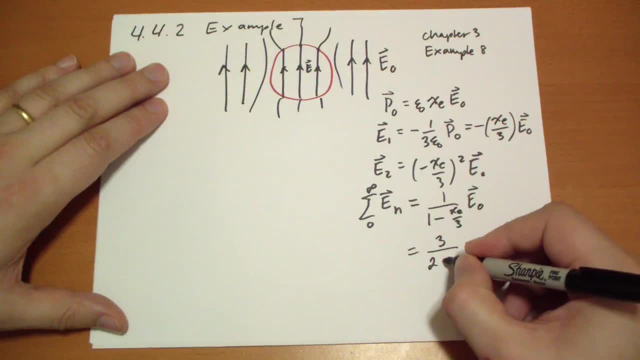 k is equal to 1 plus chi e, so that's the same as t plus k times the original electric field. so this turns out to be the resulting electric field. after doing this an infinite number of times, you get the electric field that you end up with. 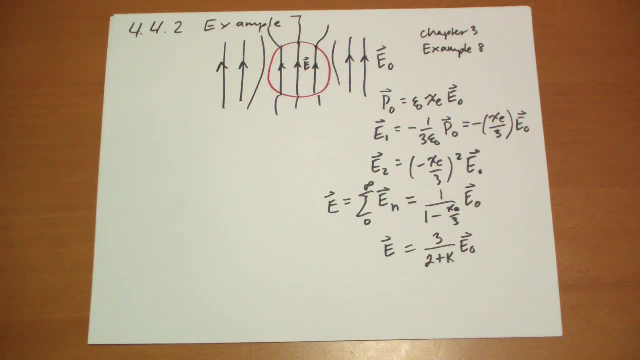 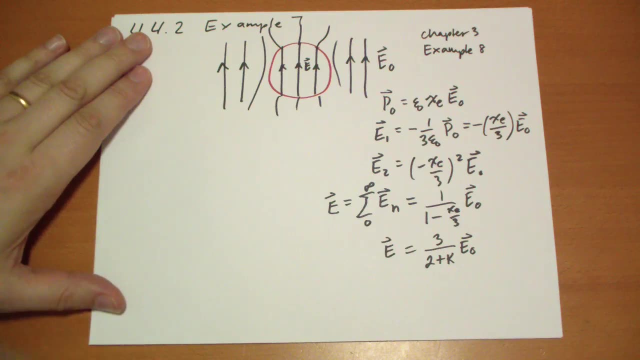 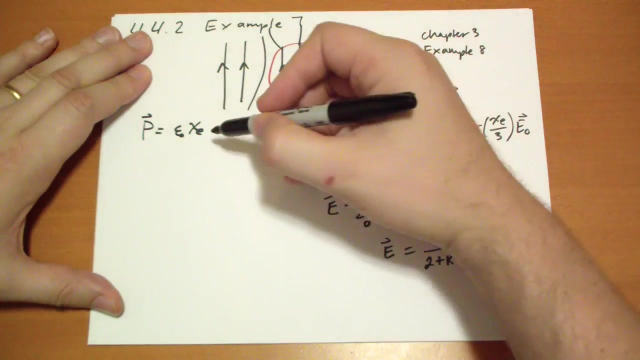 and if you're not happy with that solution, then what we can do is we can say: well, what's the resulting polarization from this electric field? so let's calculate that. so the polarization is going to be epsilon naught chi, e times the electric field we just calculated. 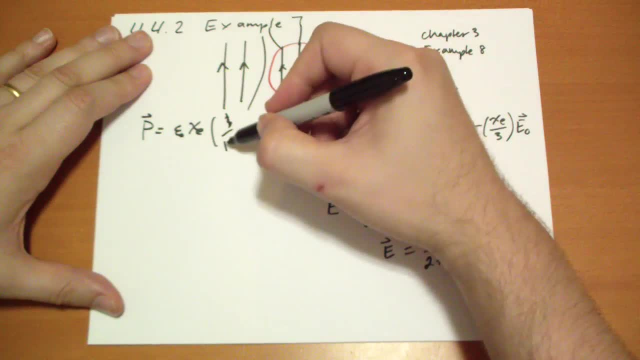 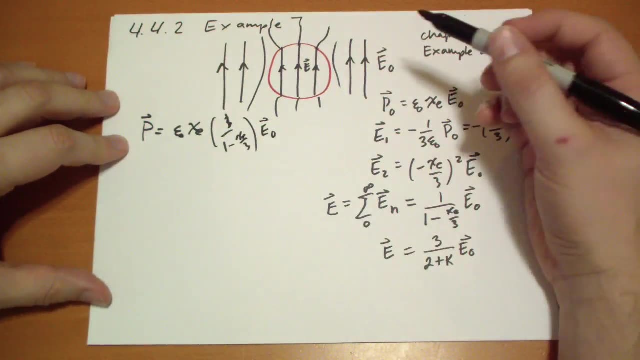 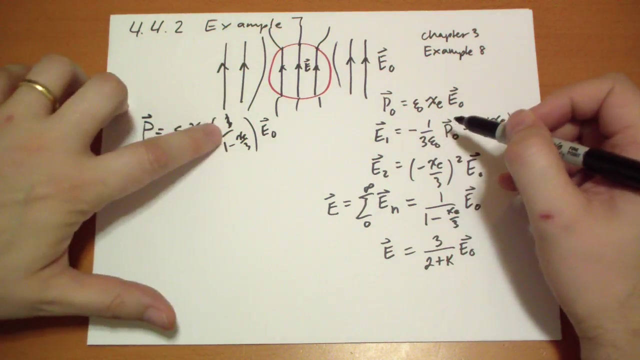 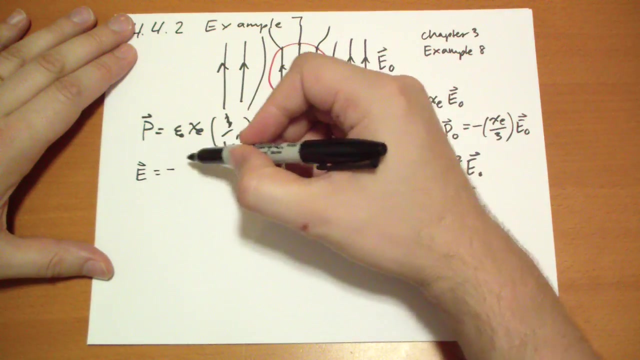 let's do 1 over 1 minus chi e over 3 times the original electric field. and what's the electric field this produces? well, that's going to be um negative 1 over 3 epsilon naught of this chunk. so that gives us negative. 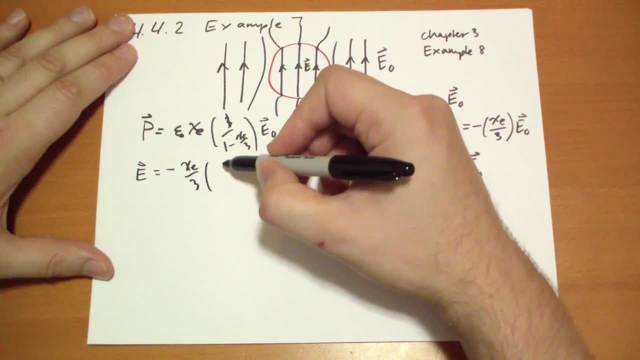 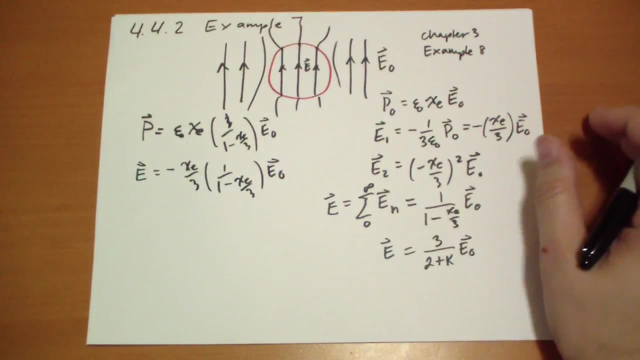 1 chi e over 3 times 1 over 1 minus chi e over 3 times the electric field. and the question is: is this the resulting electric field? does this change the field at all? so really we want to see if this is zero or non-zero or what it is. 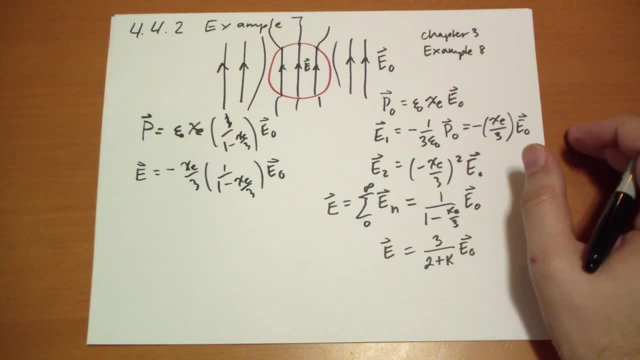 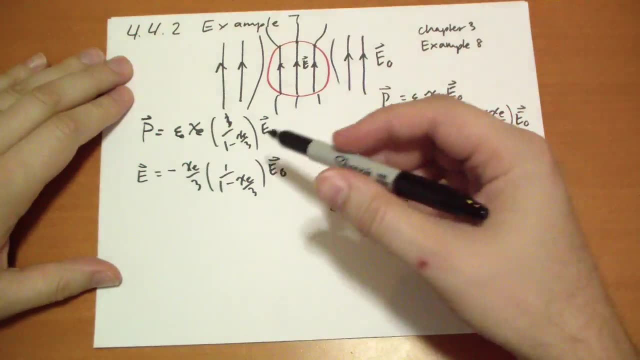 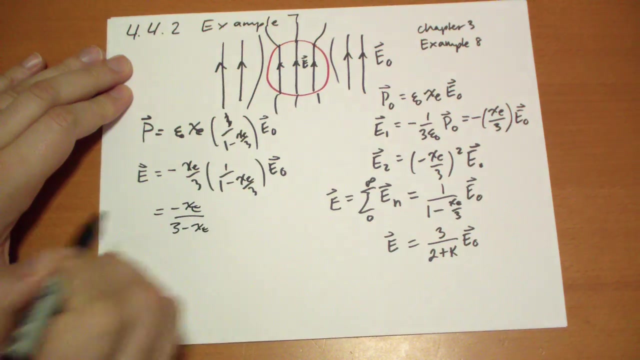 um, and so let's see how did they do this? they kind of made these numbers dance all around. so we get chi e over 3 minus chi e. so this is equal to minus chi e over 3 minus chi e, and so if we combine that with the background field, 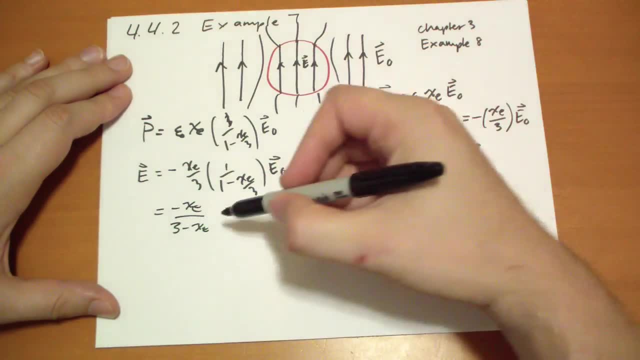 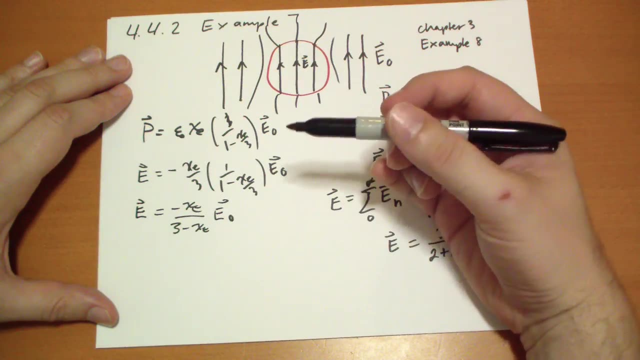 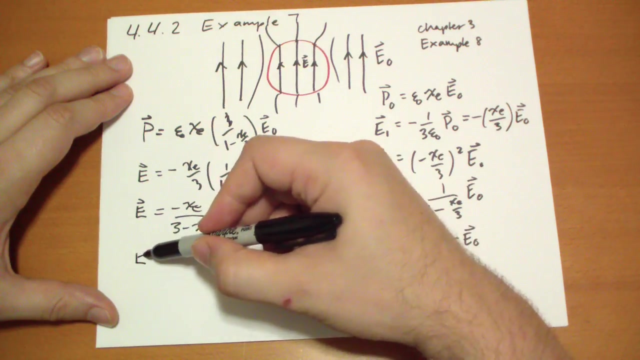 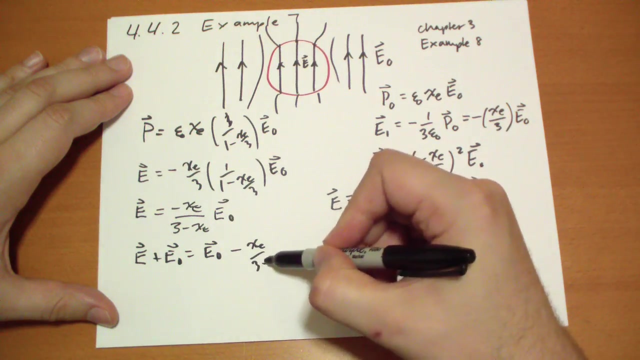 you recover the field. you recover the field you started with so, and so you add in the background field there. so the new electric field plus the electric field equals e naught minus chi, e over 3 minus chi, e epsilon naught. and that is going to be. 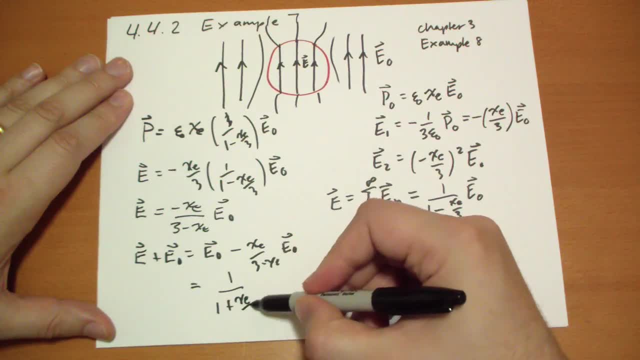 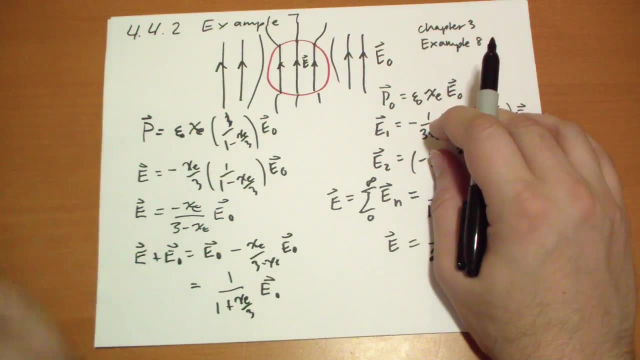 1 over 1, plus chi e over 3 of the original electric field. so the resulting electric field from adding in additional polarization due to the electric field we just calculated is basically nothing. it doesn't amount to anything. so we've kind of reached a stabilization point where 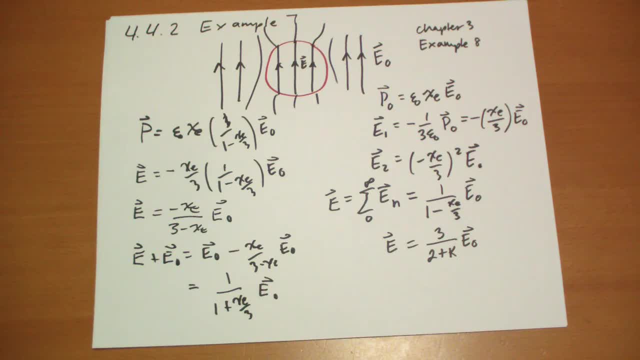 you know, doing this additional times doesn't get you any different of an answer. so the interesting thing is, this only works for spheres, it works for ellipsoids and it works for cylinders, so it doesn't work for cubes or different spheres or different shapes like that. 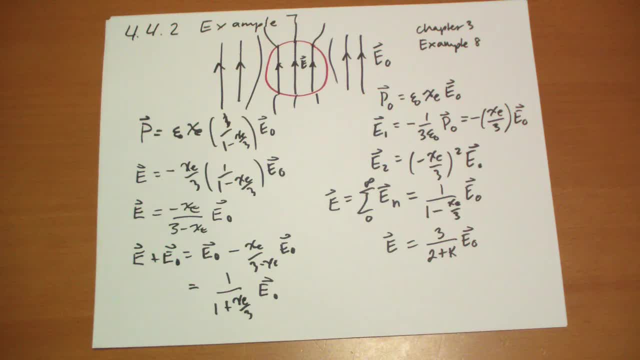 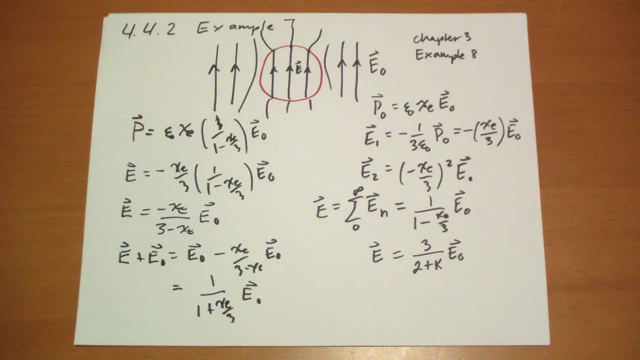 and the reason why is because as you apply the polarization due to the electric field, you get a more and more complicated field and polarization inside of the object and it's not possible to really see where it goes after applying it several times, it just becomes infinitely like a fractal.